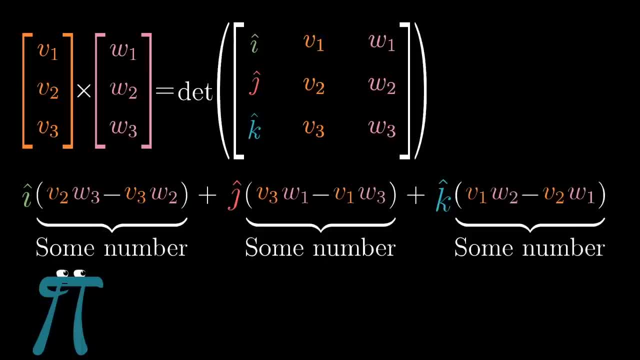 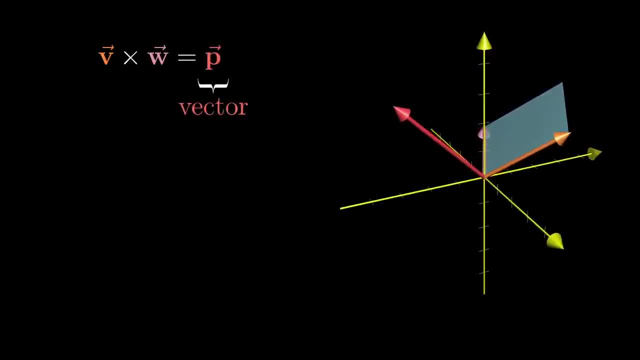 interpreted as the coordinates of some resulting vector. From here, students are typically told to just believe that the resulting vector has the following geometric properties: Its length equals the area of the parallelogram defined by v and w. It points in a direction perpendicular to both v and w. 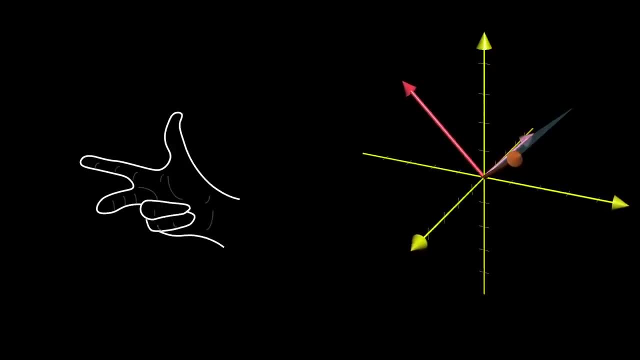 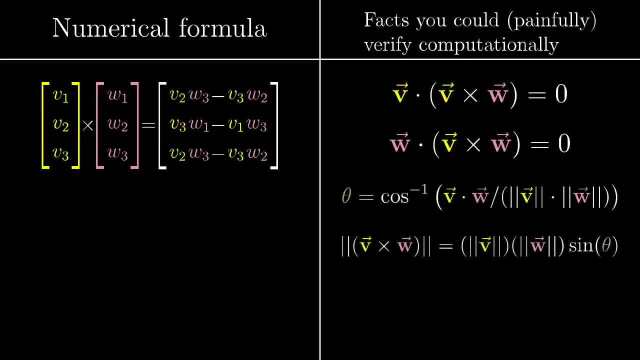 This direction obeys the right hand rule, in the sense that if you point your forefinger along v and your middle finger along w, then when you stick up your thumb it'll point in the direction of the new vector. There are some brute force computations that you could do to confirm these facts, but I 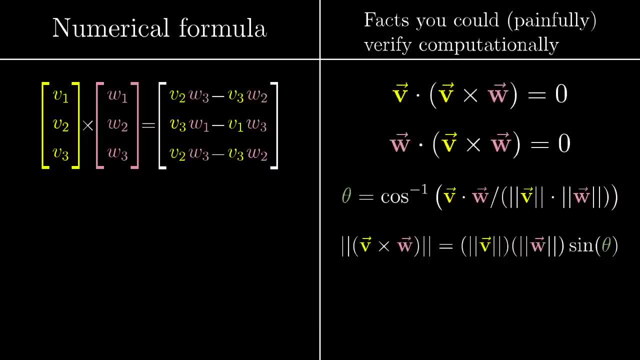 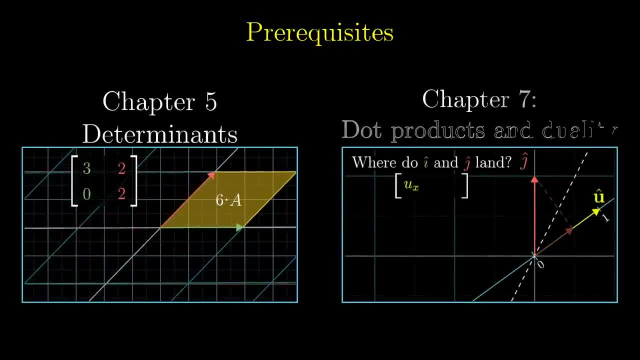 want to share with you a really elegant line of reasoning. It leverages a bit of background, though, so for this video I'm assuming that everybody has watched chapter 5, on the determinant, and chapter 7, where I introduced the idea. 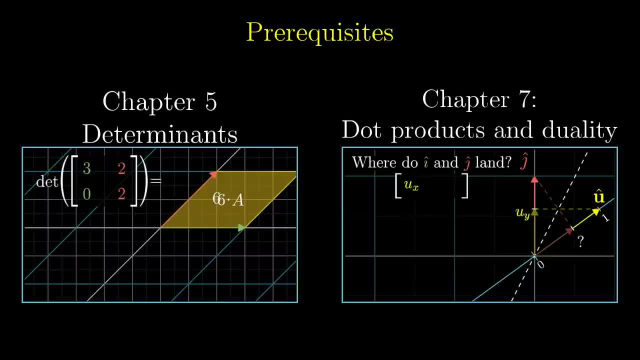 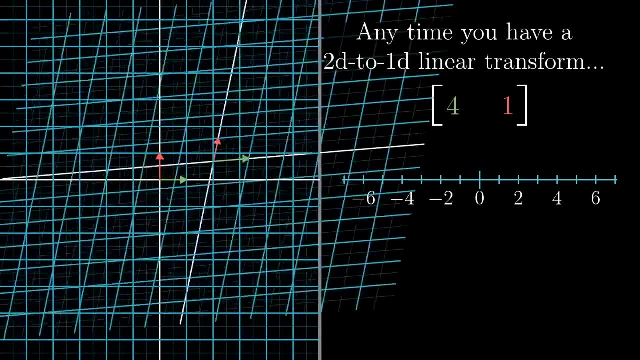 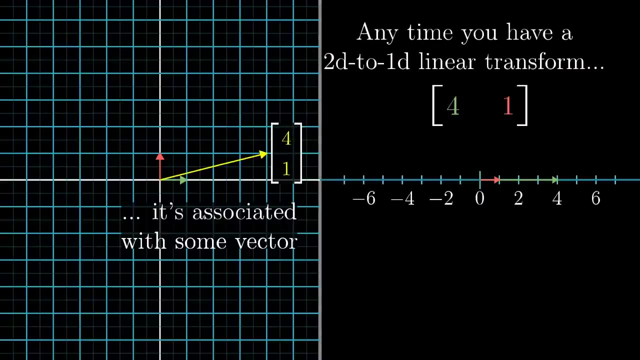 of duality. As a quick reminder, the idea of duality is that any time you have a linear transformation from some space to the number line, it's associated with a unique vector in that space, in the sense that performing the linear transformation is the same as taking a dot product with that. 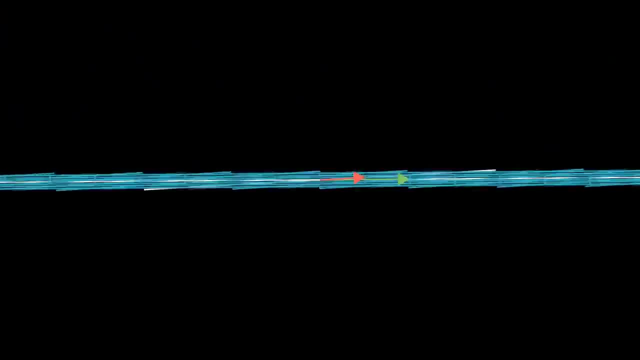 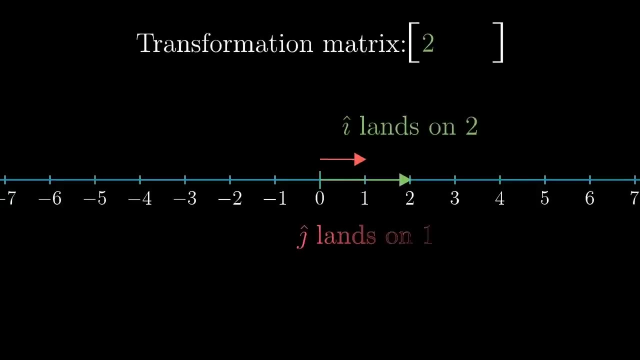 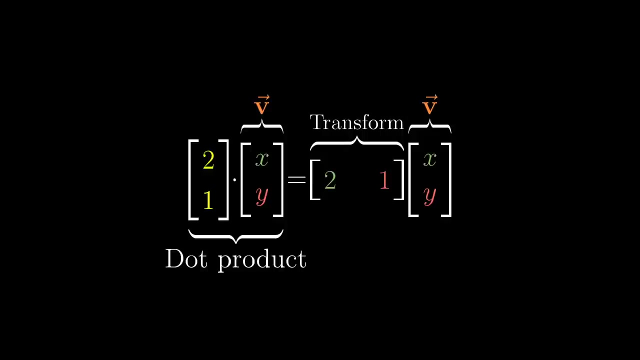 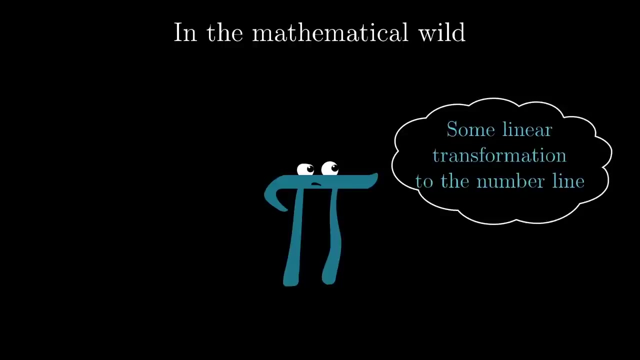 vector Numerically. this is because one of those transformations is described by a matrix with just one row. 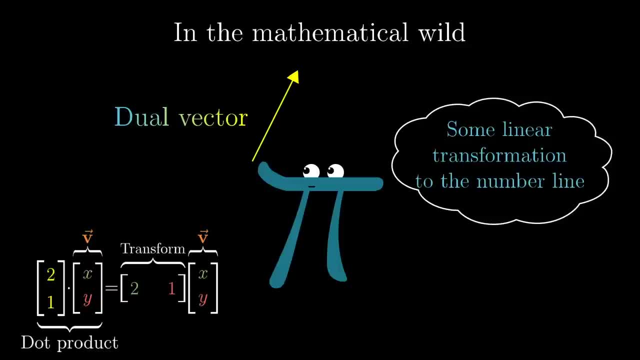 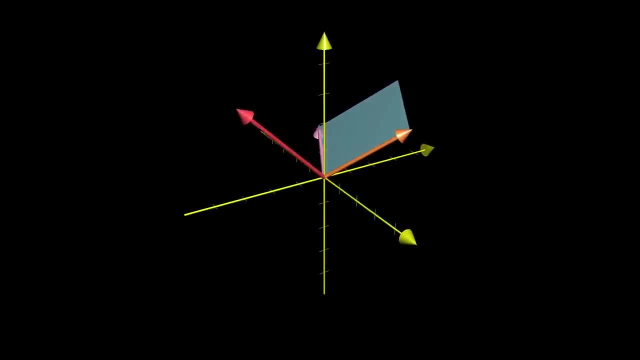 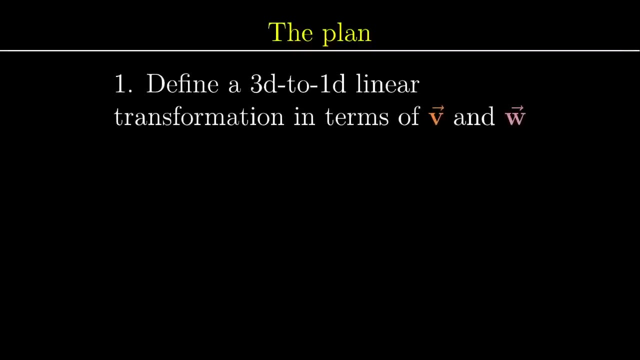 Taking the linear transformation is the same as taking a dot product with that vector. The cross product gives us a really slick example of this process in action. It takes some effort but it's definitely worth it. What I'm going to do is define a certain linear transformation from three dimensions to the. 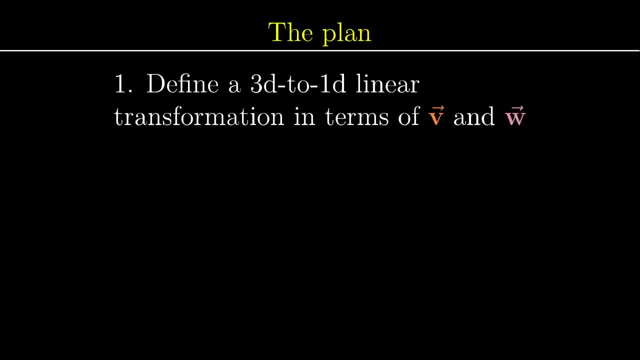 number line and it'll be defined in terms of the two vectors, v and w. Then, when we associate that transformation with its dual vector in 3D space, that dual vector is going to be the cross product of v and w. The reason for doing this will be that understanding that transformation is going to make clear 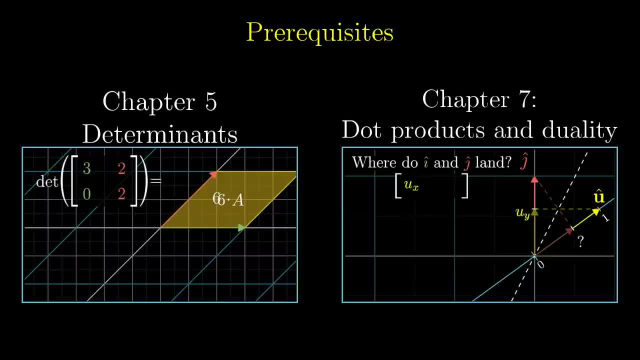 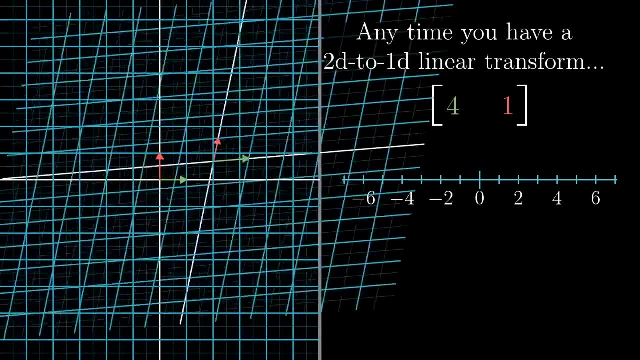 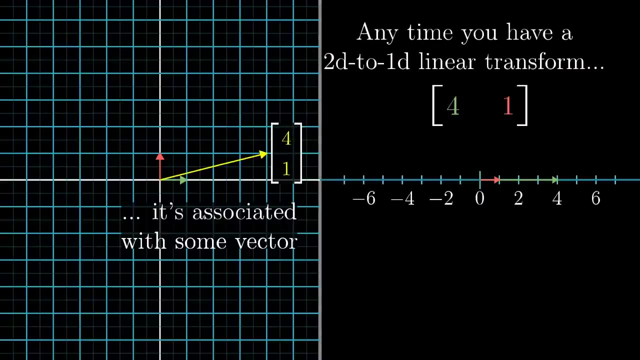 of duality. As a quick reminder, the idea of duality is that any time you have a linear transformation from some space to the number line, it's associated with a unique vector in that space, in the sense that performing the linear transformation is the same as taking a dot product with that. 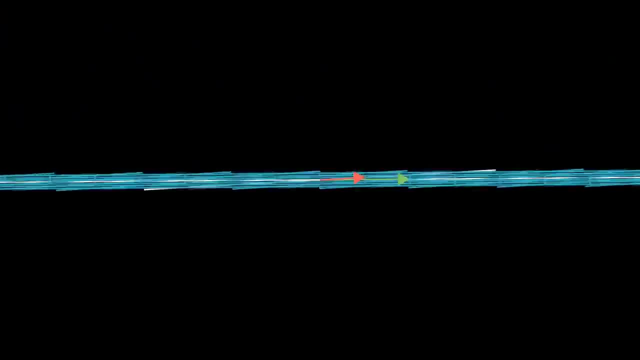 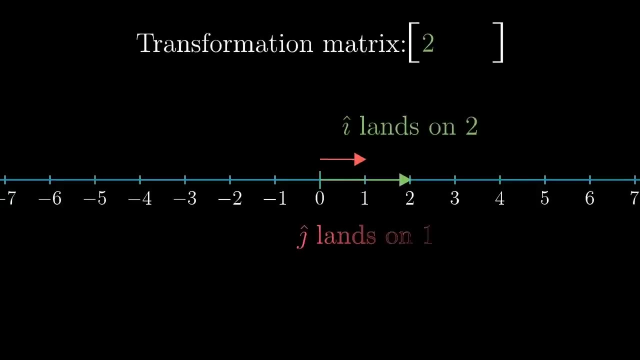 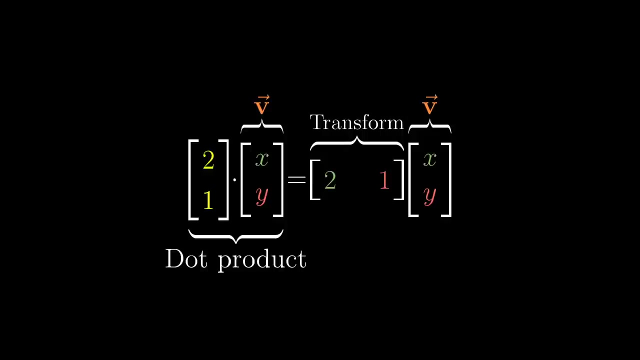 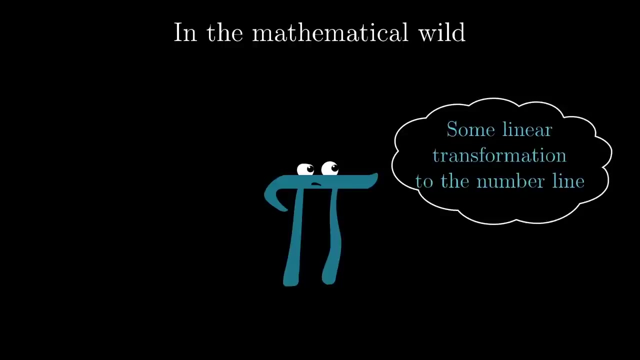 vector Numerically. this is because one of those transformations is described by a matrix with just one row. 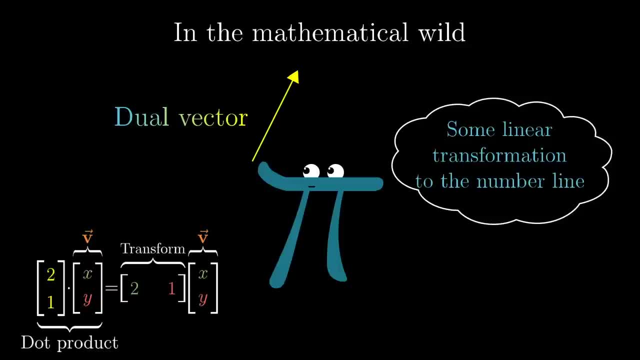 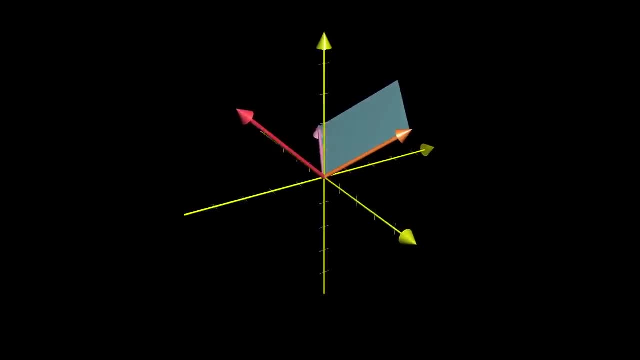 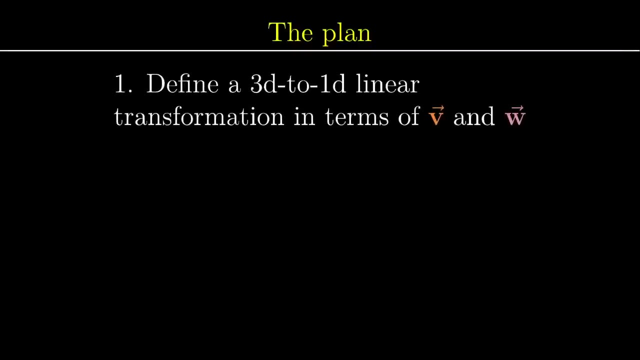 The cross product gives us a really slick example of this process in action. It takes some effort, but it's definitely worth it. What I'm going to do is define a certain linear transformation from three dimensions to the number line, and it will be defined in terms of the two vectors v and w. 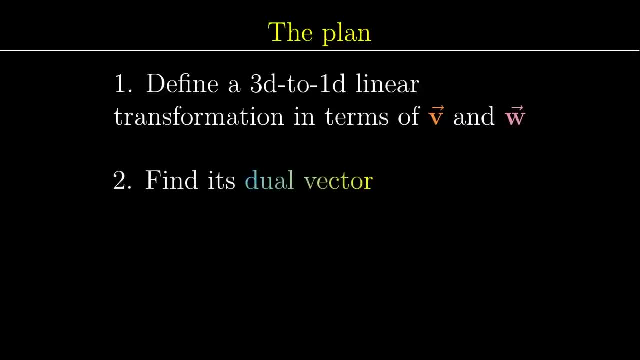 Then when we associate that transformation with its dual vector in 3D space, that dual vector is going to be the cross product of v and w. The reason for doing this will be that understanding that transformation is going to make clear the connection between: 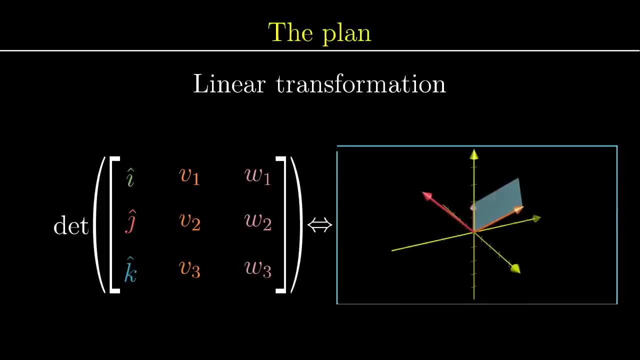 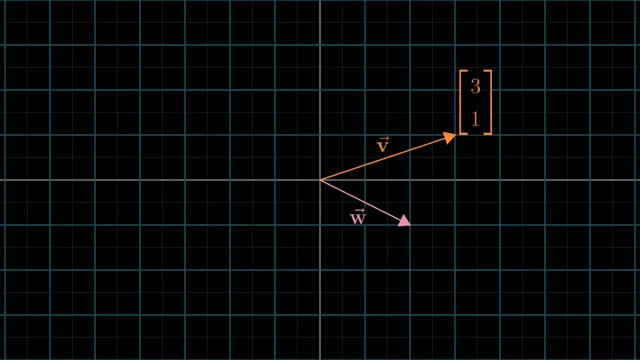 the computation and the geometry of the cross product. So to back up a bit, remember in two dimensions what it meant to compute the 2D version of the cross product. When you have two vectors, v and w, you put the coordinates of v as the 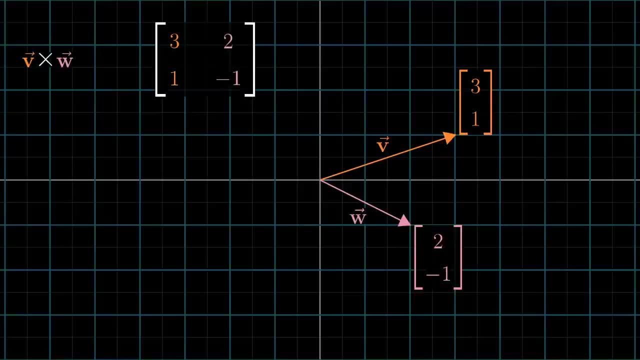 first column of a matrix and the coordinates of w as the second column of a matrix. Then you just compute the determinant. There's no nonsense with basis vectors stuck in a matrix or anything like that, just an ordinary determinant returning a number Geometrically. 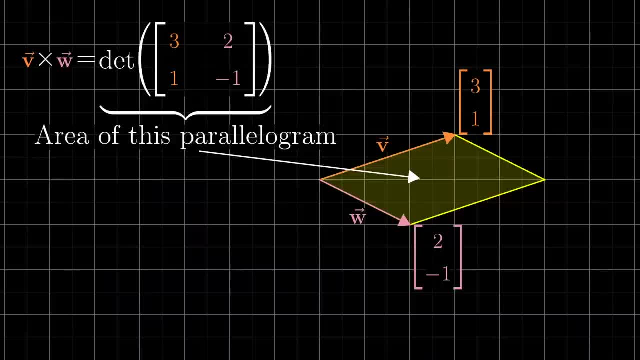 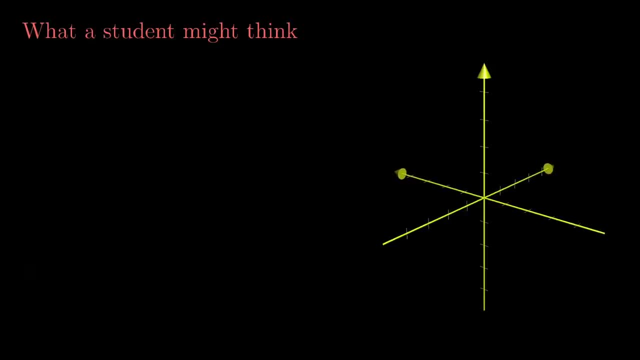 this gives us the area of a parallelogram spanned out by those two vectors, with the possibility of being negative depending on the orientation of the vectors. Now, if you didn't already know the 3D cross product and you're trying to extrapolate, you might imagine. 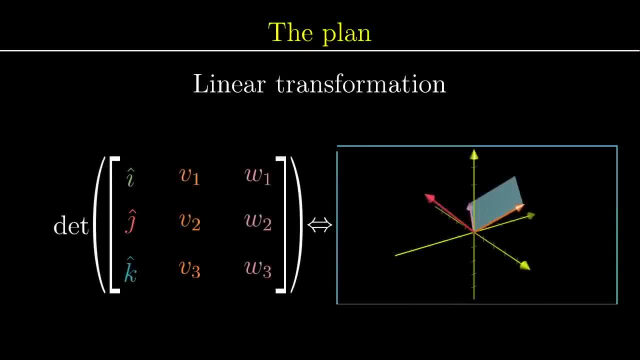 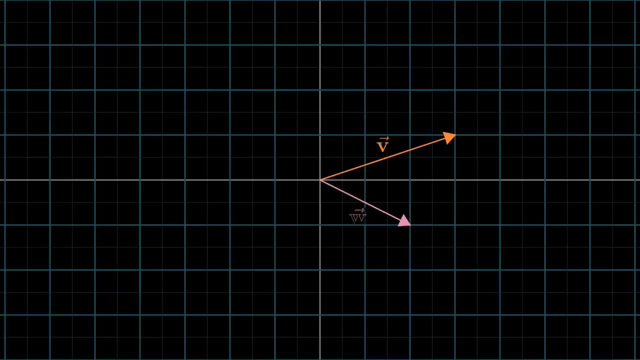 the connection between the computation and the geometry of the cross product. So to back up a bit, remember in two dimensions what it meant to compute the 2D version of the cross product. When you have two vectors, v and w, You put the coordinates of v as the first column of a matrix and the coordinates of 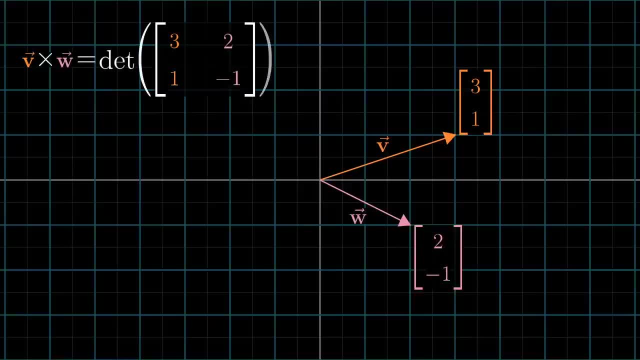 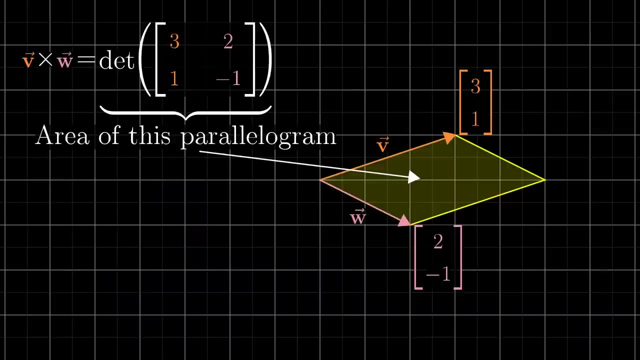 w as the second column of a matrix, then you just compute the determinant. There's no nonsense with basis vectors stuck in a matrix or anything like that, just an ordinary determinant returning a number Geometrically. this gives us the area of a parallelogram spanned out by those two vectors. 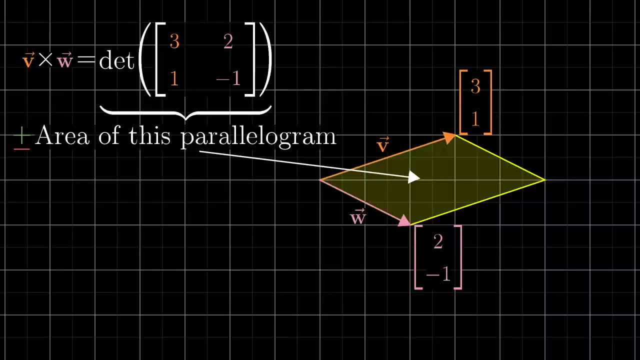 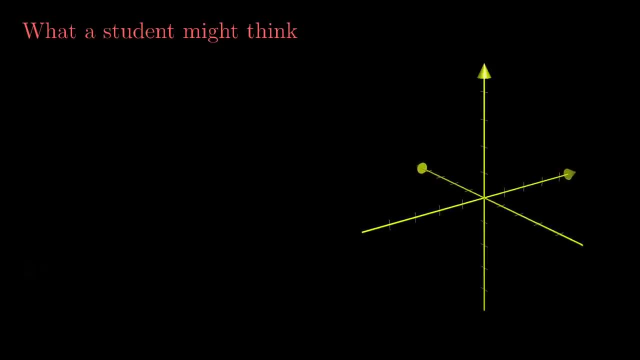 with the possibility of being negative depending on the orientation of the vectors. Now, if you didn't already know the 3D cross product and you're trying to extract and extrapolate, you might imagine that it involves taking three separate 3D vectors. 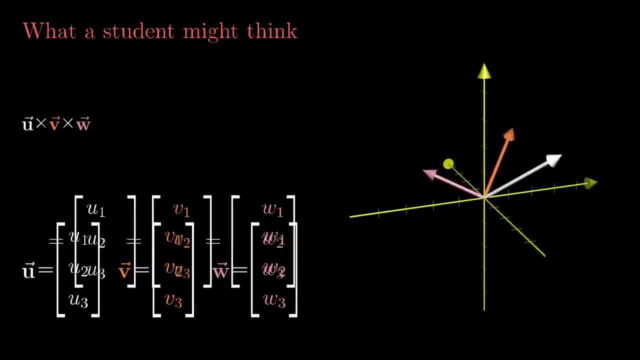 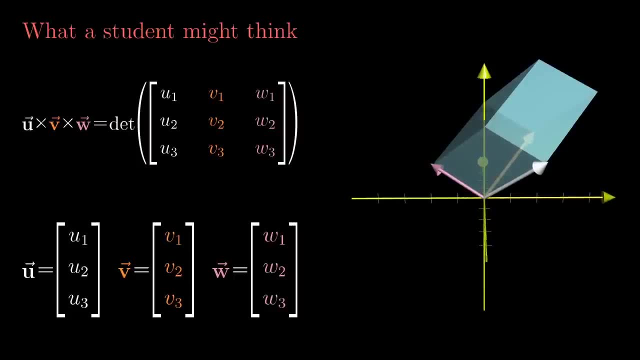 u, v and w and making their coordinates the columns of a 3x3 matrix, then computing the determinant of that matrix And, as you know from chapter 5,, geometrically this would give you the volume of a parallelepiped. 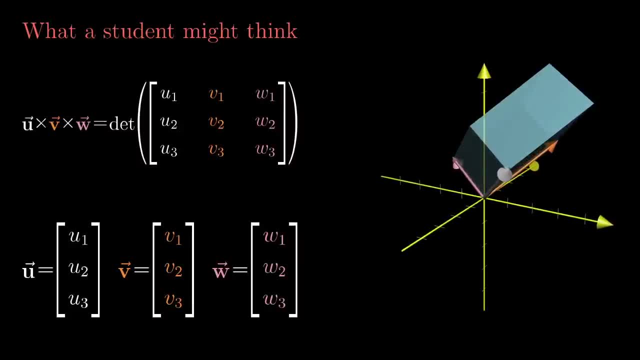 spanned out by those three vectors with a plus or minus sign depending on the right-hand rule orientation of those three vectors. Of course, you all know that this is not the 3D cross product. The actual 3D cross product takes in two vectors and spits out a vector. 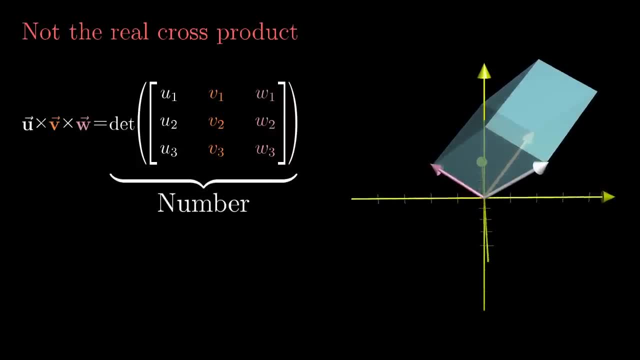 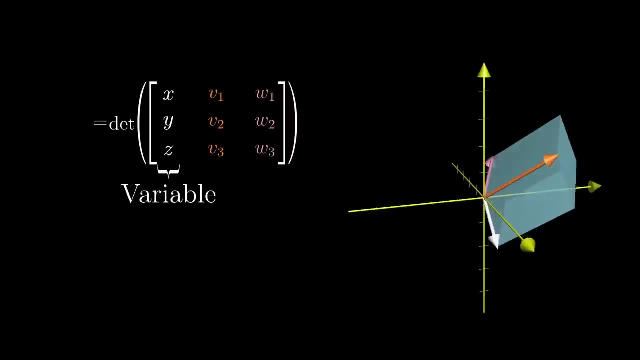 It doesn't take in three vectors and spit out a number, But this idea actually gets us really close to what the real cross product is. Consider that first vector, u, to be a variable, say with variable entries x, y and z, while 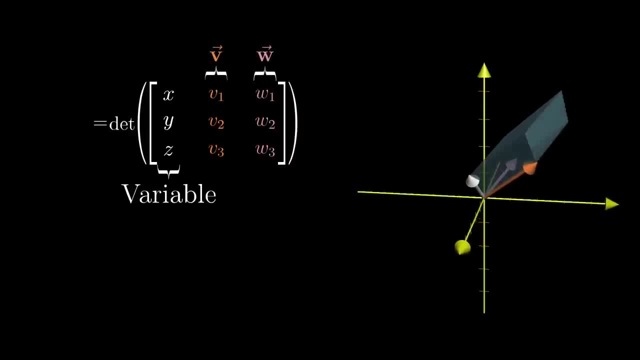 v and w remain fixed. What we have, then, is a function from three dimensions to the number line. You input some vector- x, y, z- and you get out a number by taking the determinant of a matrix whose first column is x, y, z and whose other two columns are the coordinates. 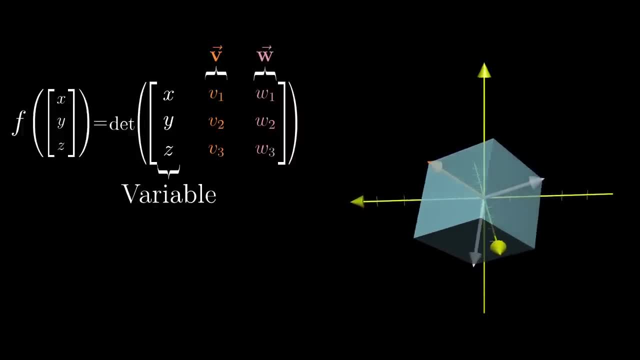 of the constant vectors v and w Geometrically. the meaning of this function is that for any input vector x, y, z- you consider the parallelepiped defined by this vector v and w, Then you return its volume. 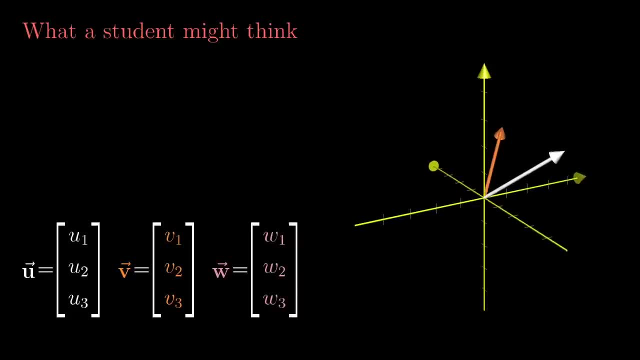 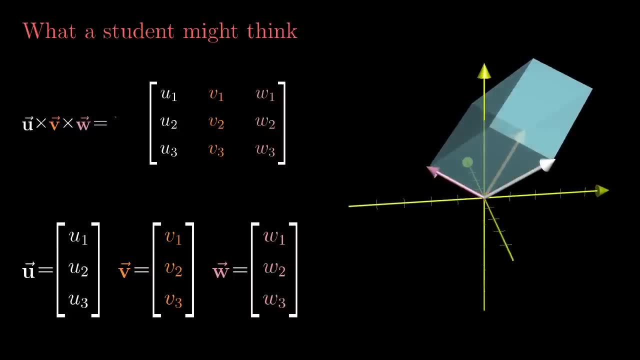 that it's going to be a cross product of a 3D cross product and you're trying to extrapolate. but it involves taking three separate 3D vectors- u, v and w- and making their coordinates the columns of a 3x3 matrix, then computing the determinant of that matrix And, as you 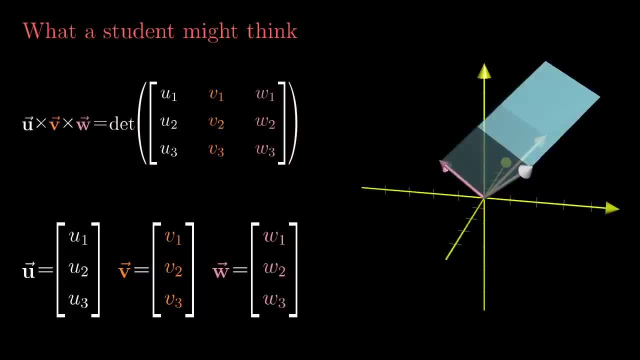 know from chapter 5, geometrically, this would give you the volume of a parallelepiped spanned out by those three vectors, with a plus or minus sign depending on the right hand rule orientation of those three vectors. Of course you all know that this is not the 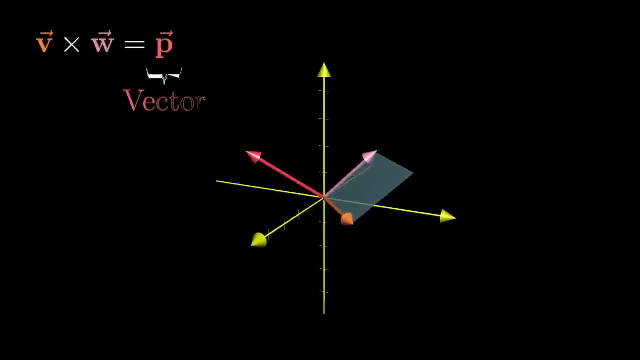 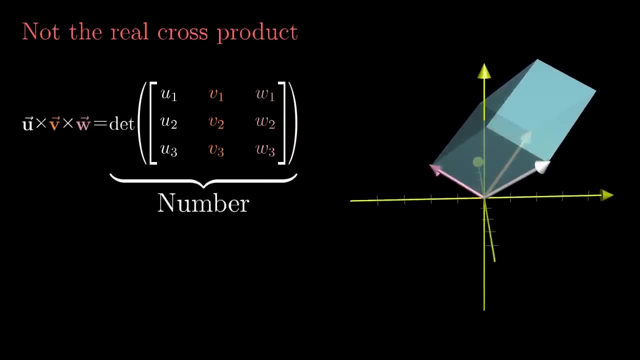 3D cross product. The actual 3D cross product takes in two vectors and spits out a vector. It doesn't take in three vectors and spit out a number. But this idea actually gets us really close to what the real cross product is. Consider that first vector, u, to be a variable. 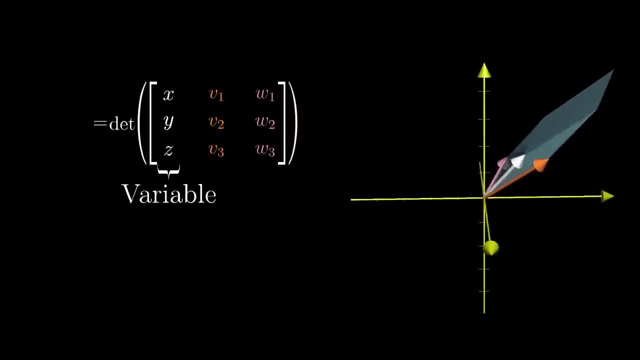 say, with variable entries x, y and z, while v and w remain fixed. What we have then is a function to be a variable. This is the same function from three dimensions to the number line. You input some vector- x, y and z- and you get out a number by taking the determinant of a matrix whose first column 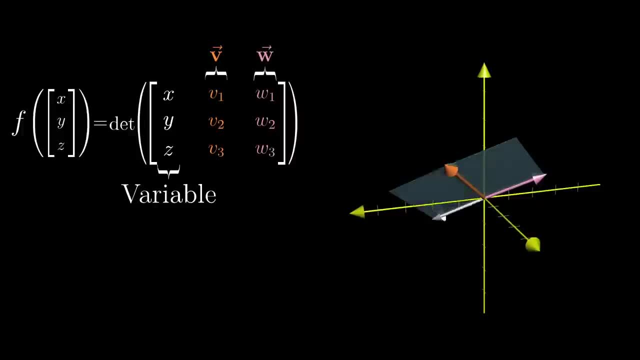 is x, y and z and whose other two columns are the coordinates of the constant vectors v and w Geometrically. the meaning of this function is that for any input vector x, y and z, you consider the parallelepiped defined by this vector v and w, then you return its. 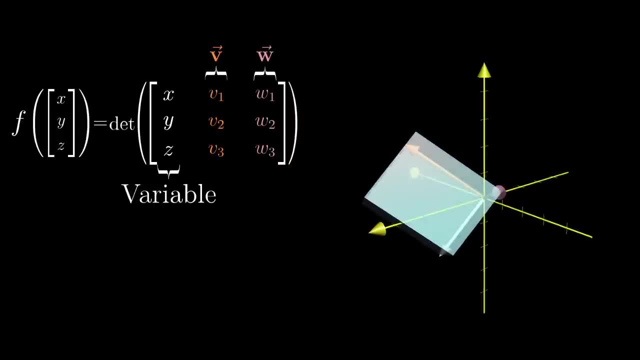 volume, With a plus or minus sign depending on orientation. This is the same function as before, but with a plus or minus sign depending on orientation. Now, this might feel like kind of a random thing to do. I mean, where does this function? 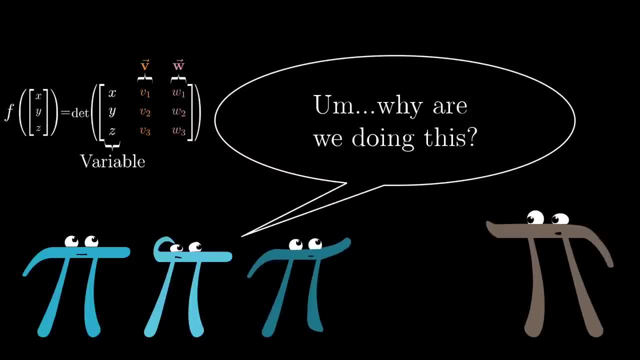 come from. Why are we defining it this way? And I'll admit, at this stage it might kind of feel like it's coming out of the blue, But if you're willing to go along with it and play around with the properties that this guy has, it's the key to understanding the 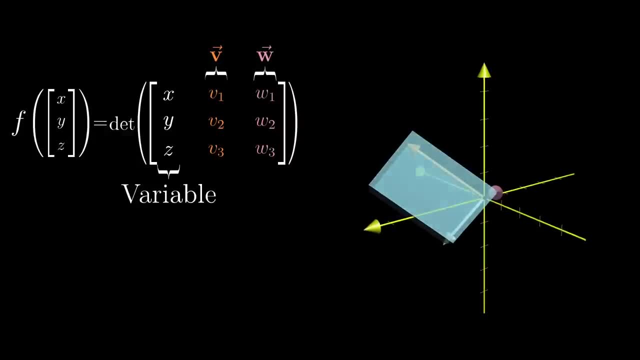 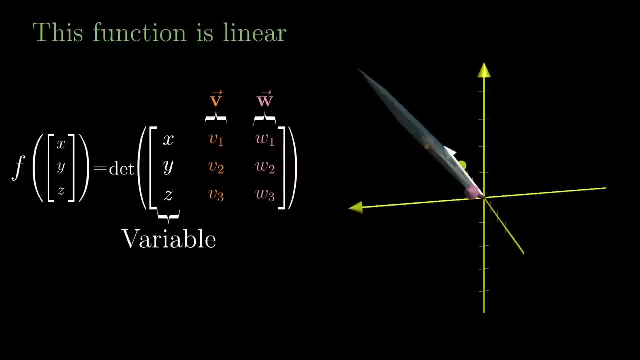 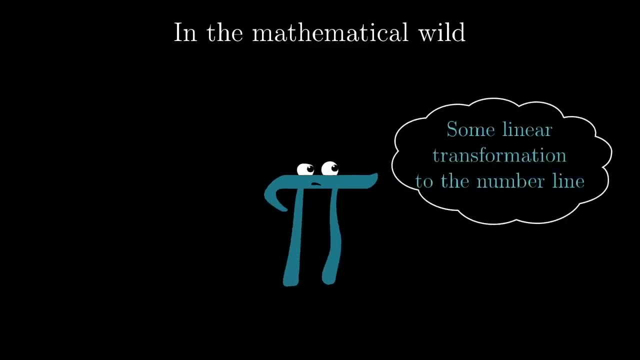 cross product. One really important fact about this function is that it's linear. I'll actually leave it to you to work through the details of why this is true, based on properties of the determinant, But once you know that it's linear, we can start bringing in the idea of duality Once. 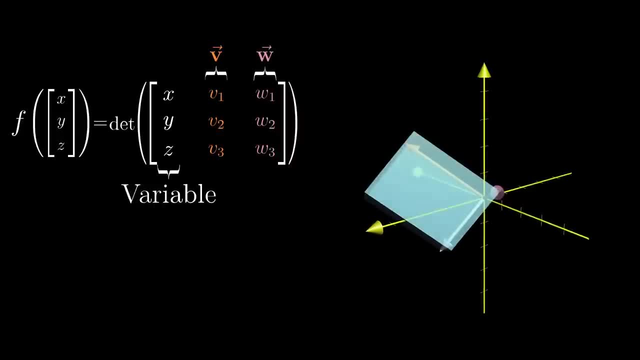 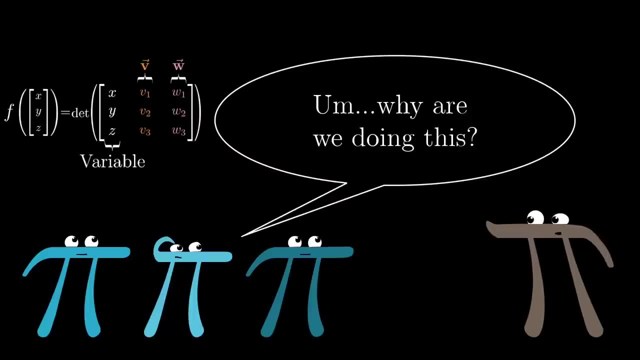 With a plus or minus sign depending on orientation. Now this might feel like kind of a random thing to do. I mean, where does this function come from? Why are we defining it this way? And I'll admit, at this stage it might kind of feel like it's coming out of the blue. 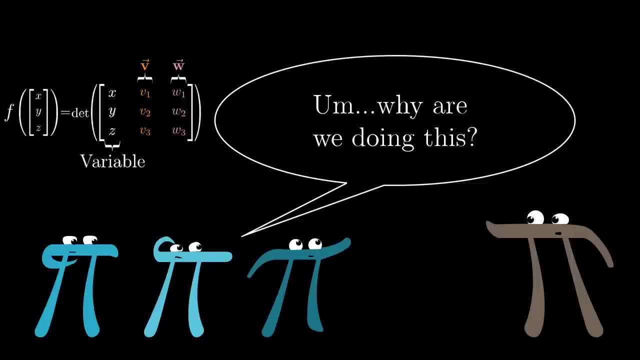 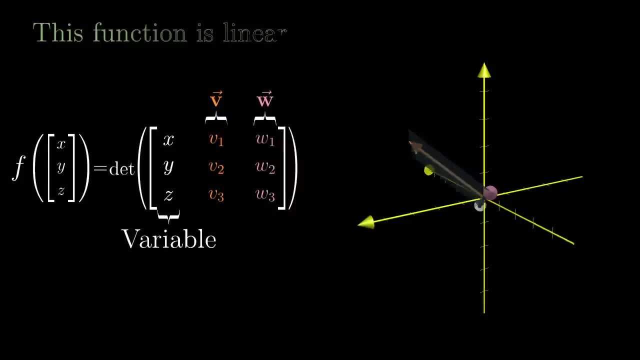 But if you're willing to go along with it and play around with the properties that this guy has, it's the key to understanding the cross product. One really important fact about this function is that it's linear. I'll actually leave it to you to work through the details of why this is true. 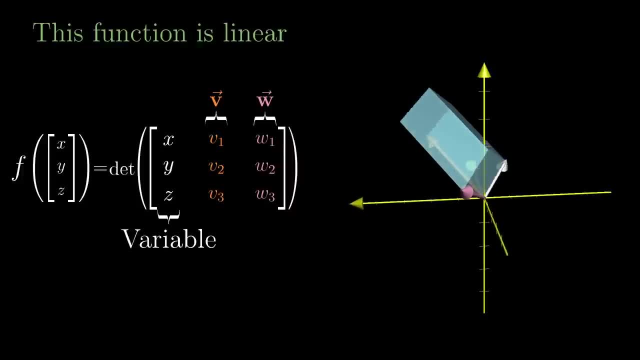 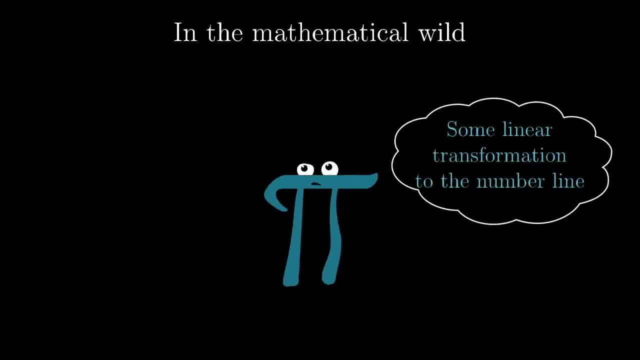 I'll leave it to you to work through the details of why this is true. I'll leave it to you to work through the details of why this is true, based on properties of the determinant. But once you know that it's linear, we can start bringing in the idea of duality. 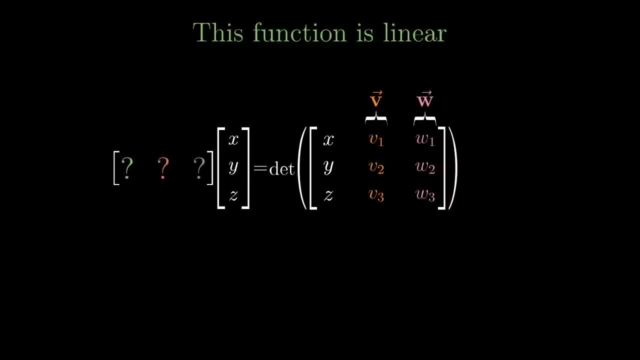 Once you know that it's linear, you know that there's some way to describe this function as matrix multiplication. Specifically, since it's a function that goes from three dimensions to one dimension, there will be a 1 by 3 matrix that encodes this transformation. 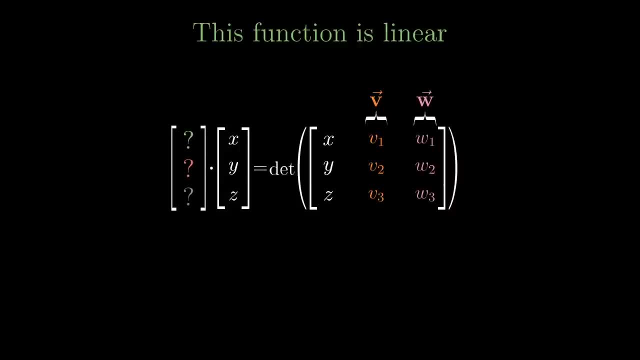 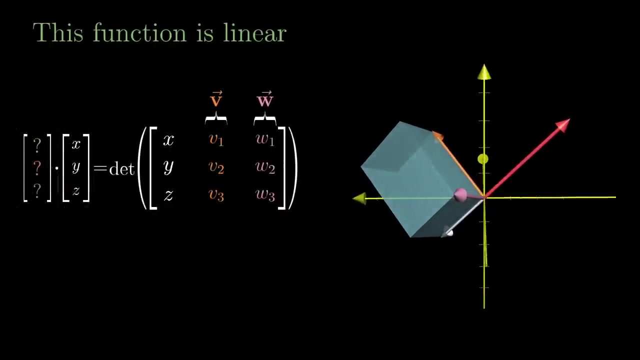 And the whole idea of duality is that the special thing about transformations from several dimensions to one dimension is that you can turn that matrix on its side and instead interpret the entire transformation as the dot product with a certain vector. What we're looking for is the special 3D vector that I'll call p, such that, taking the dot, 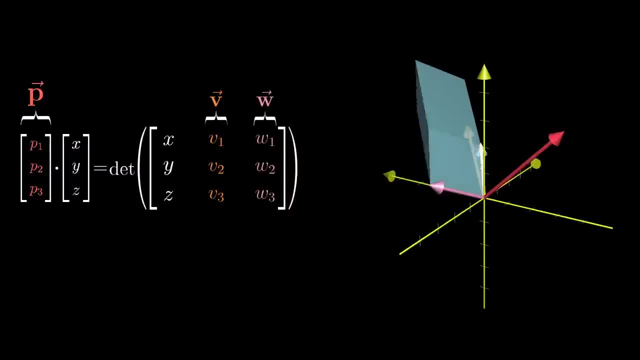 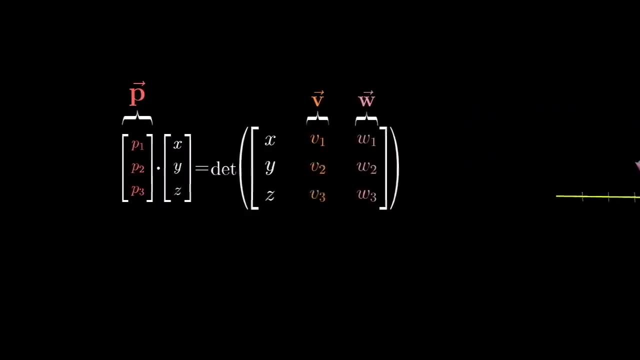 product between p and any other vector. x y z gives the same result as plugging in x y z as the first column of a 3 by 3 matrix, And that's the whole idea of duality. I'll get to the geometry of this in just a moment, but right now let's dig in and think. 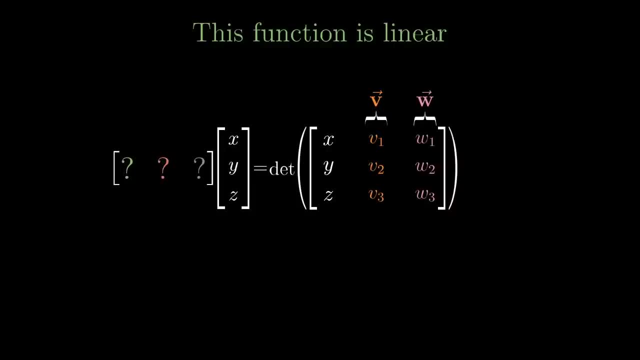 you know that it's linear. you know that there's some way to describe this function as matrix multiplication, Specifically, since it's a function that goes from three dimensions to one dimension, there will be a 1 by 3 matrix that encodes this transformation And the 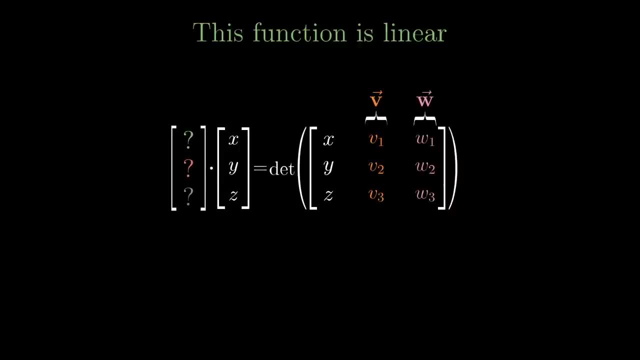 whole idea of duality is that it's linear. The idea of duality is that the special thing about transformations from several dimensions to one dimension is that you can turn that matrix on its side and instead interpret the entire transformation as the dot product with a certain vector. What we're looking for is 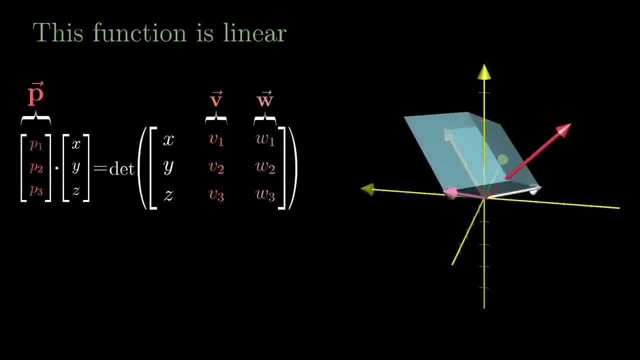 the special 3D vector that I'll call p, such that taking the dot product between p and any other vector, x y z- gives the same result as plugging in x y z as the first column of a 3 by 3 matrix whose other two columns are the same. So what we're looking for is: 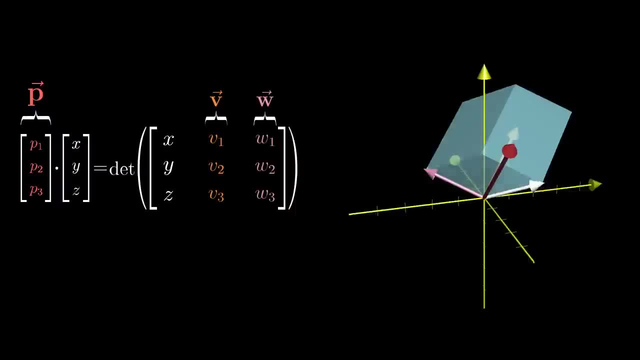 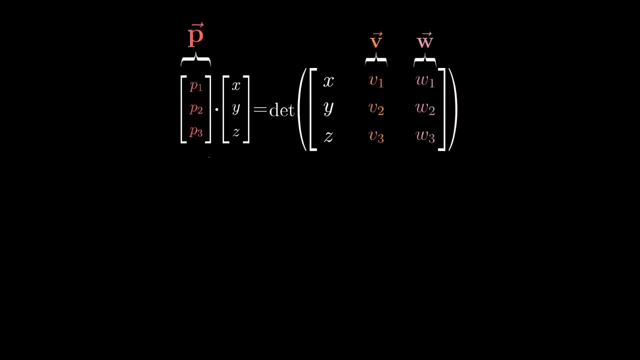 that the two columns have the coordinates of v and w, then computing the determinant. I'll get to the geometry of this in just a moment, but right now let's dig in and think about what this means computationally. Taking the dot product between p and x, y, z will: 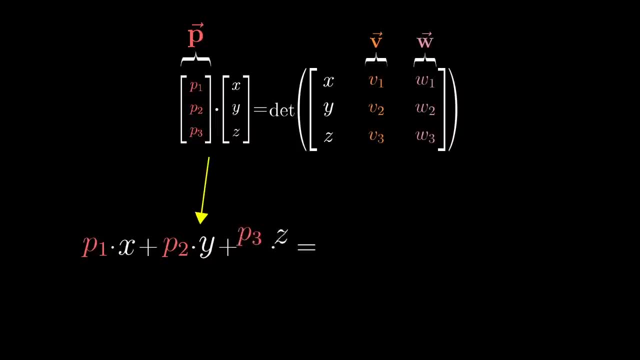 give us something times x plus something times y plus something times z, where those somethings are the coordinates of p. But on the right side here, when you compute the determinant, you can organize it to look like some constant times x plus some constant times y plus some. 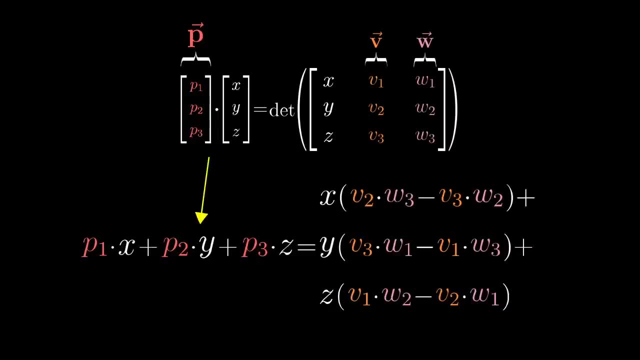 constant times z, where those constants involve certain combinations of the components of v and w. So those constants, those particular combinations of the coordinates of v and w, are going to be the coordinates of the vector p that we're looking for. But what's going? 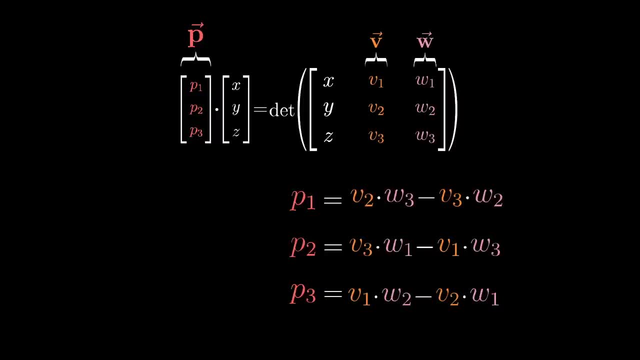 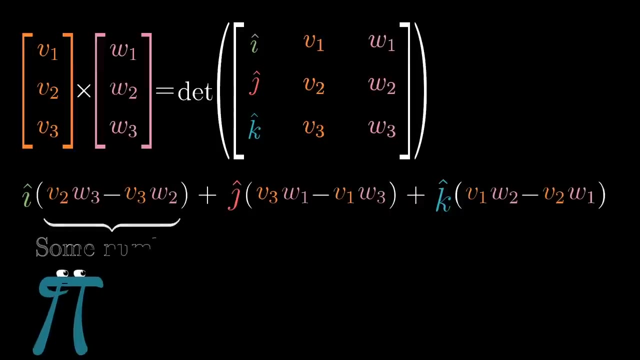 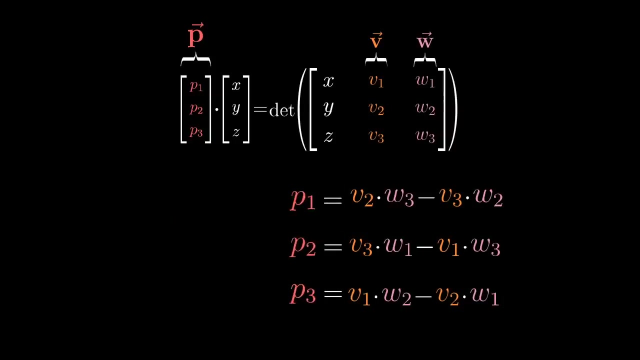 on on the right here should feel very familiar to anyone who's actually worked through a cross product computation. So what we're going to do is we're going to take the dot product, then the dot product, we're going to take the vector and we're going to multiply that by some non-sthartistic 연습. Let's Alliance. 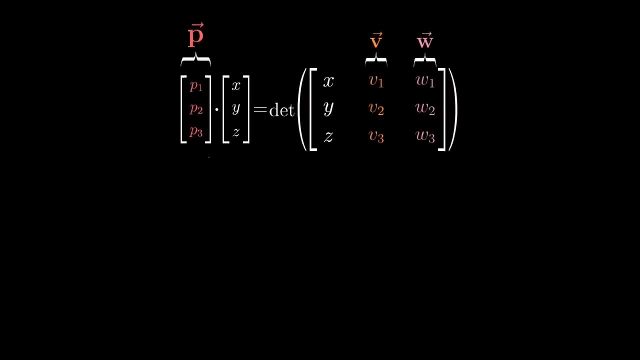 about what this means computationally. Taking the dot product between p and x y z will give us something times x plus something times y plus something times z, where those somethings are the coordinates of p. But on the right side here, when you compute the determinant, you can organize it to look. 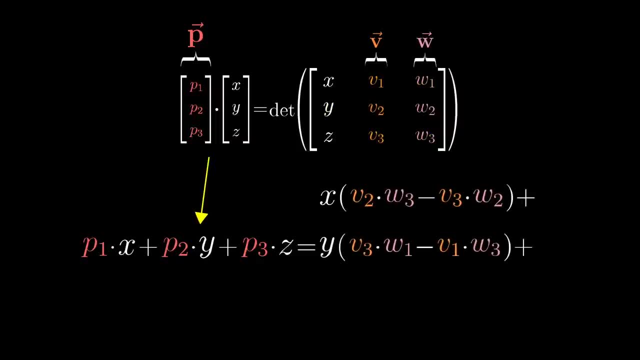 like some constant. So we have some constant times x plus some constant times y, plus some constant times z, where those constants involve certain combinations of the components of v and w. So those constants, those particular combinations of the coordinates of v and w, are going to 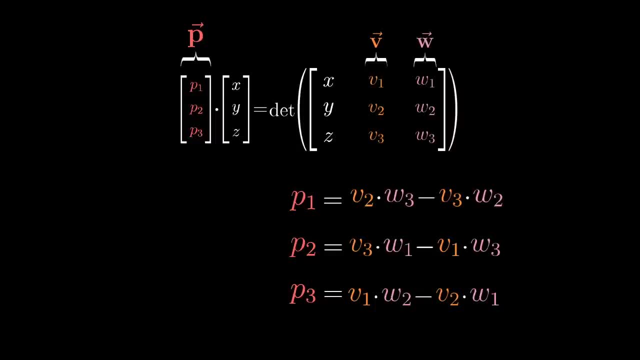 be the coordinates of the vector p that we're looking for. But what's going on on the right here should feel very familiar to anyone who's actually doing a cross product computation. Collecting the constant terms that are multiplied by x, y and z like this is no different from 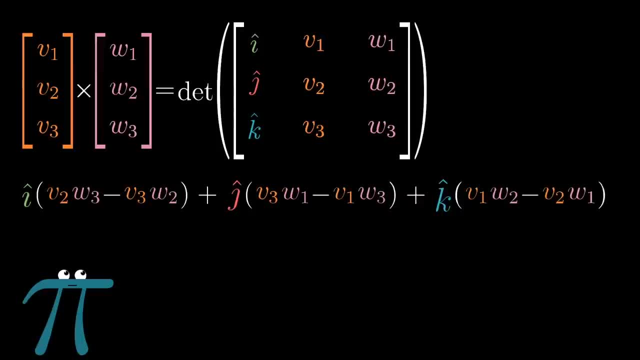 plugging in the symbols i-hat, j-hat and k-hat to that first column and seeing which coefficients aggregate on each one of those terms. It's just that plugging in i-hat, j-hat and k-hat is a way of signaling that we should 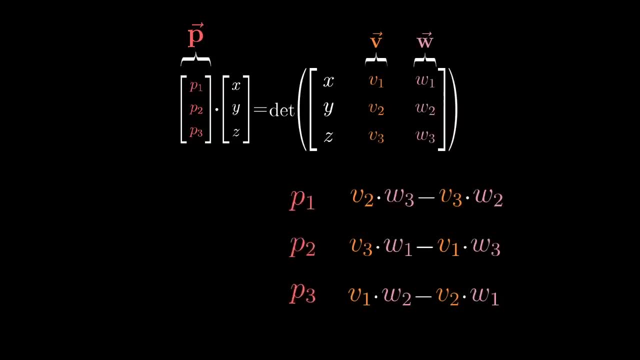 interpret those coefficients as the coordinates of a vector. So what all of this is saying is that the next step is to essentially come up with a displacement function. And that's what that 2 by 2 matrix puzzle does. It's just that we'll нек to a fraction and we'll get to the constant value of a. 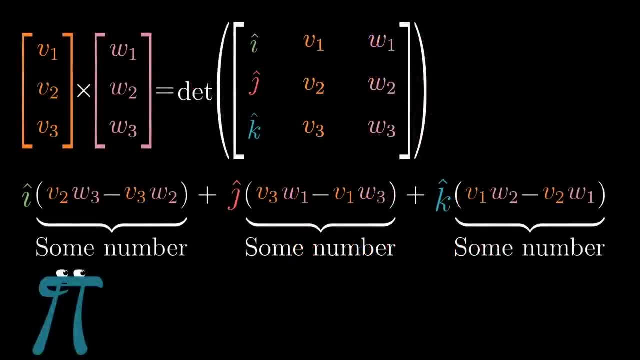 2 by 2 matrix. The next step is to make a column of p and you can look for the coordinates of that vector. So what this is saying is that the one that we have to do is to multiply each one of the. But this funky computation can be thought of as a way to answer the following question. 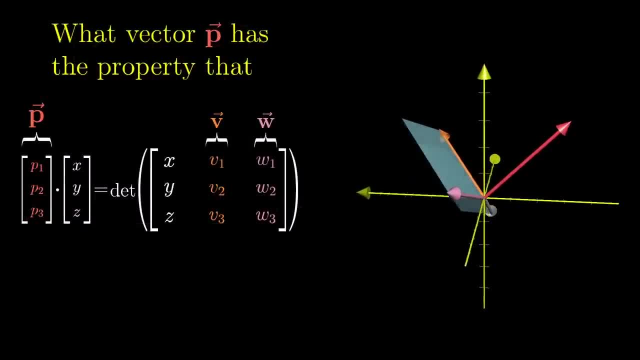 What vector p has the special property that when you take a dot product between p and some vector x, y, z, it gives the same result as plugging in x, y, z to the first column of a matrix whose other two columns have the coordinates of v and w, then computing. 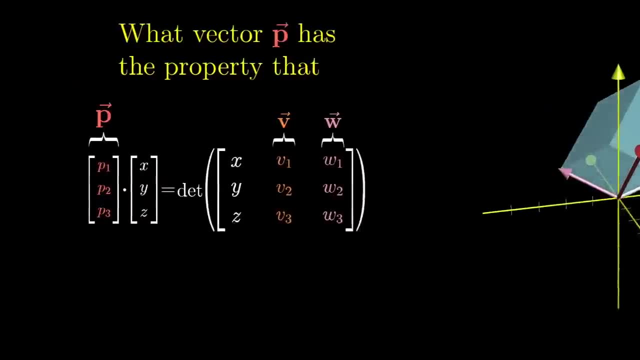 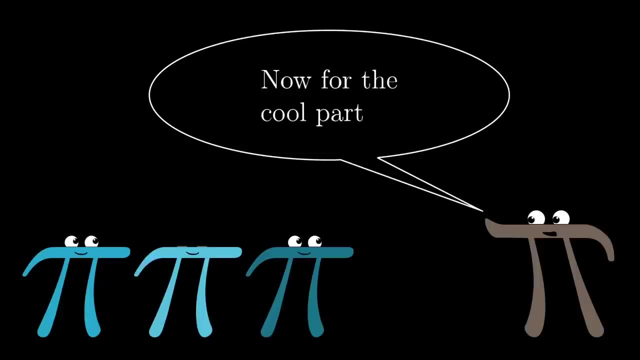 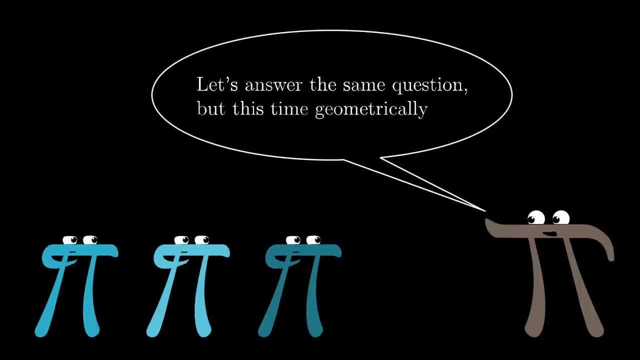 the determinant? That's a bit of a mouthful, but it's an important question to digest for this video. Now for the cool part which ties all this together with the geometric understanding of the cross product that I introduced last video. I'm going to ask the same question again, but this time we're going to try to answer. 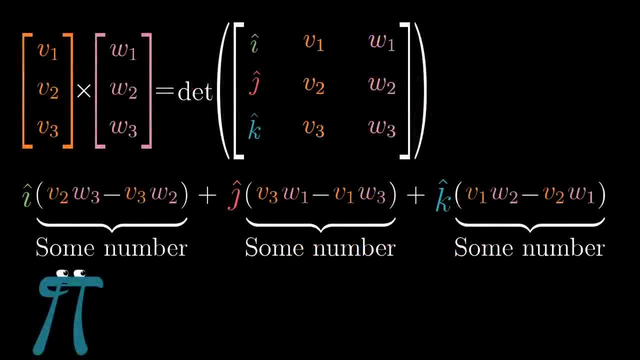 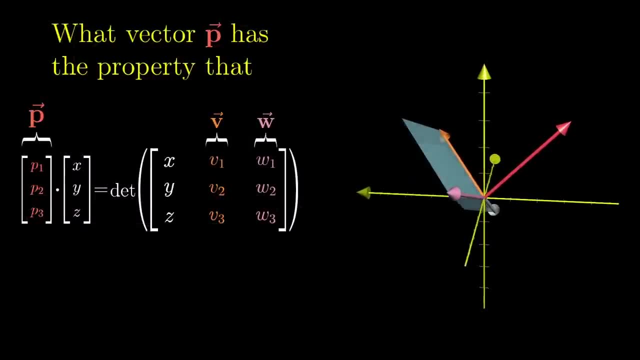 the zeros. However, I don't think ALL of this is going to work. It's going to be a fantasy. This funky computation can be thought of as a way to answer the following question: What vector p has the special property that when you take a dot product between p and 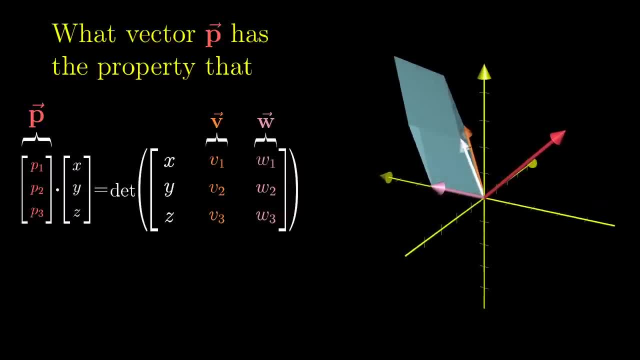 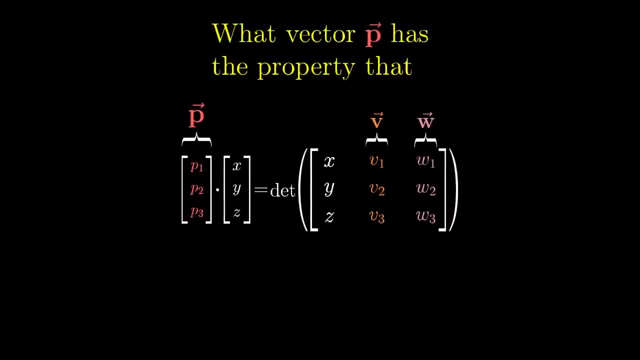 some vector, x, y, z. it gives the same result as plugging in x, y, z to the first column of a matrix whose other two columns have the coordinates of v and w, then computing the determinant. That's a bit of a mouthful, but it's an important question to digest for this video. 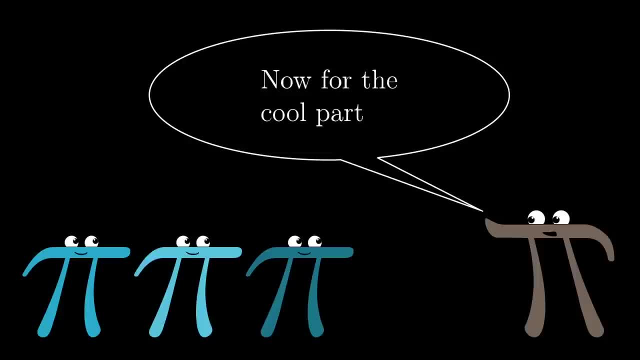 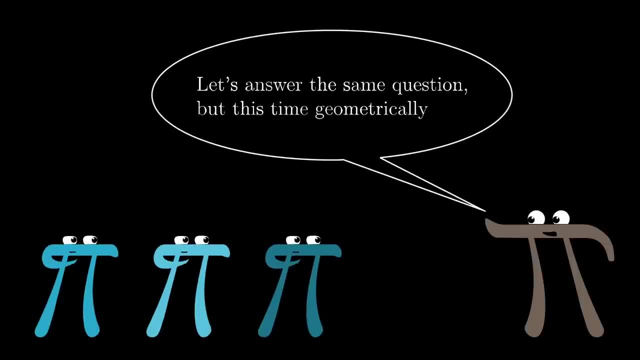 Now for the cool part, which ties all this together with the geometric understanding of the cross product that I introduced last video. I'm going to ask the same question again, but this time we're going to try to answer it geometrically instead of computationally. 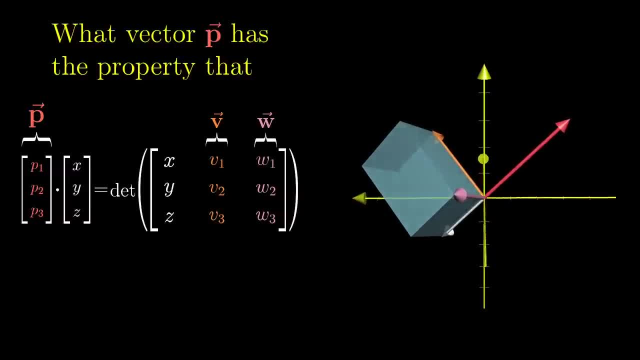 What 3D vector p has the special property that when you take a dot product between p and some other vector x, y, z, it gives the same result as if you took the signed volume of a parallelepiped defined by this vector x, y, z to the first column of a matrix. 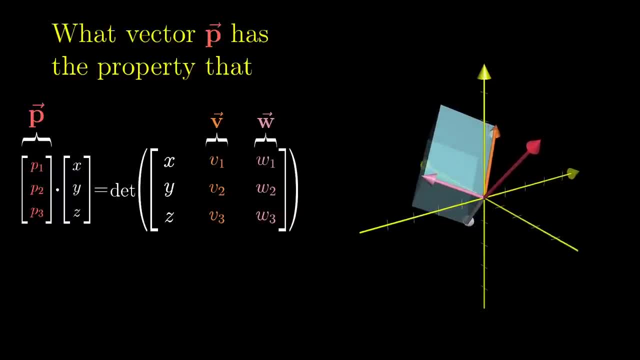 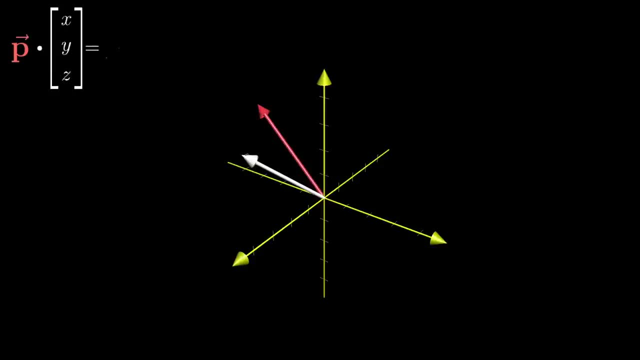 x, y, z, along with v and w. Remember the geometric interpretation of a dot product between a vector, p and some other vector is to project that other vector onto p, then to multiply the length of that projection by the length of p. 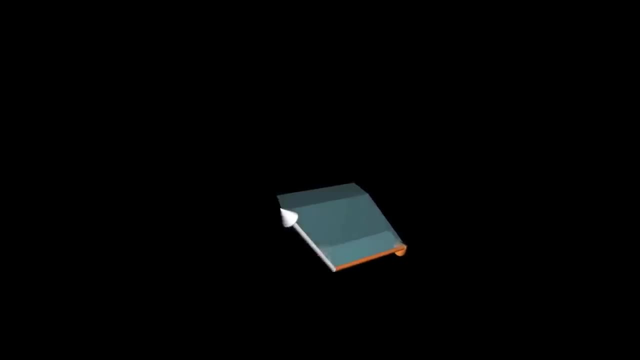 With that in mind, let me show a certain way to think about the volume of the parallelepiped that we care about. Start by taking the area of the vector x y z, along with v and w, Then multiply it not by the length of x y z, but by the component of x y z, that's. 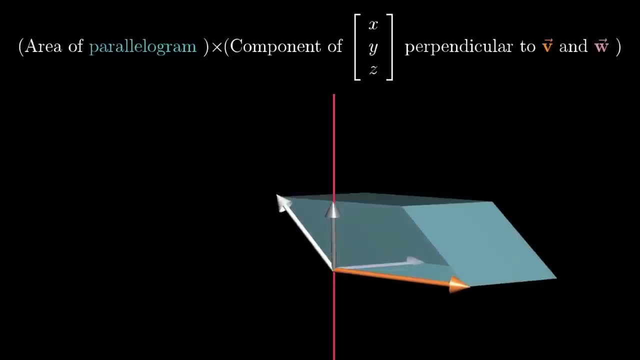 perpendicular to that parallelepiped. In other words, the way our linear function works on a given vector is to project that vector onto a line that's perpendicular to both v and w, then to multiply the length of that projection by the area of the parallelepiped spanned by v and w. 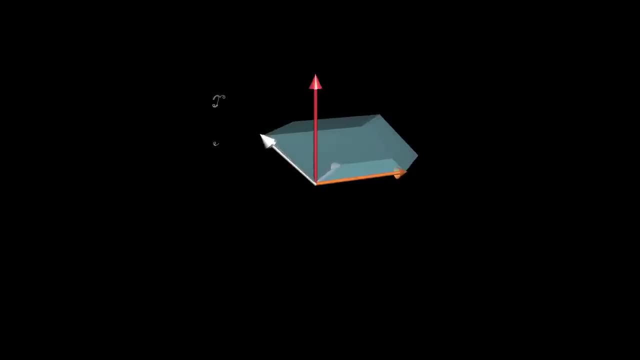 But this is the same thing as taking a dot product between xyz and a vector that's perpendicular to v and w with a length equal to the area of the parallelogram. What's more, if you choose the appropriate direction for that vector, the cases where 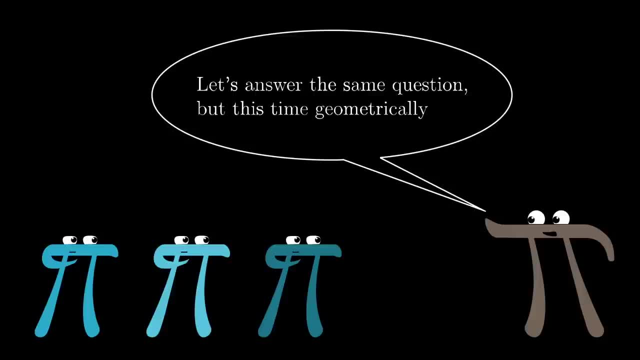 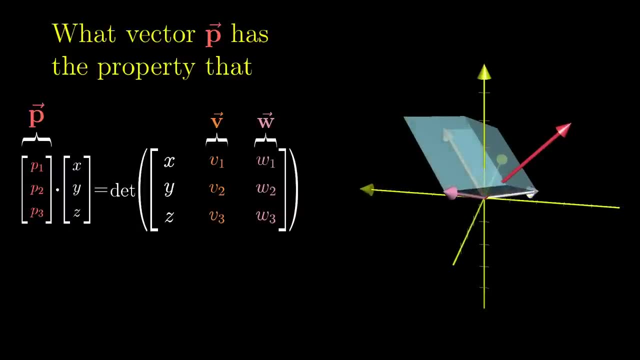 it geometrically instead of computationally. What 3D vector p has the special property that when you take a dot product between p and some other vector x, y, z- it gives the same result as if you took the signed volume of a parallelepiped defined by this vector x y, z to the first column of a matrix. 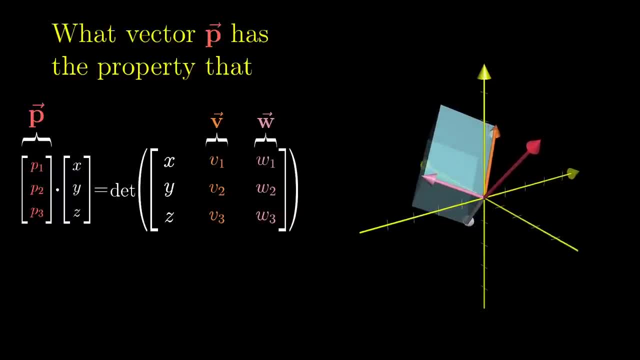 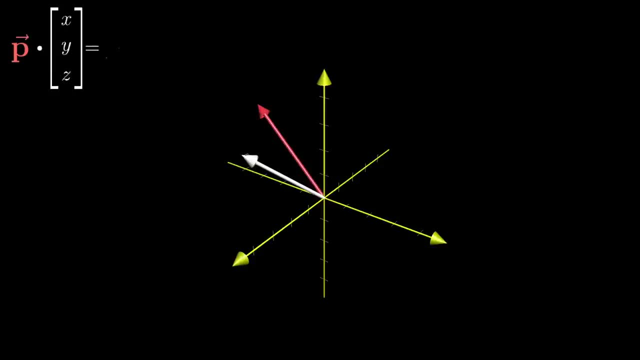 x, y, z, along with v and w. Remember the geometric interpretation of a dot product between a vector, p and some other vector is to project that other vector onto p, then to multiply the length of that projection by the length of p. 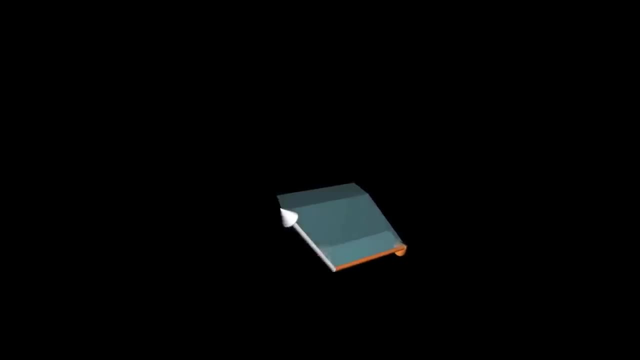 With that in mind, let me show a certain way to think about the volume of the parallelepiped that we care about. Start by taking the area of the vector x y z, along with v and w, Then multiply it not by the length of x y z, but by the component of x y z, that's. 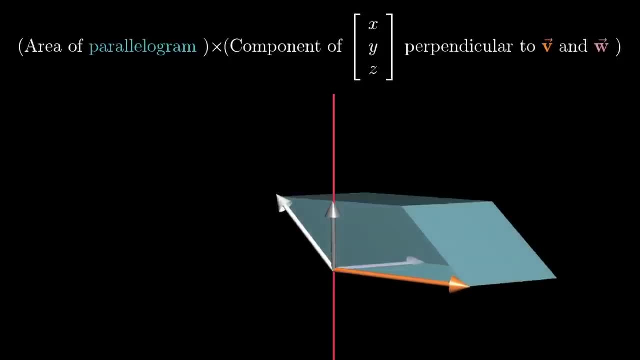 perpendicular to that parallelepiped. In other words, the way our linear function works on a given vector is to project that vector onto a line that's perpendicular to both v and w, then to multiply the length of that projection by the area of the parallelepiped spanned by v and w. 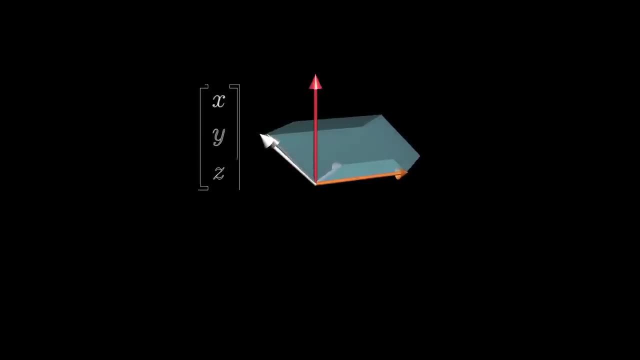 But this is the same thing as taking a dot product between x, y, z and a vector that's perpendicular to v and w, with a length equal to the area of that parallelogram. What's more, if you choose the appropriate direction for that vector, the cases where 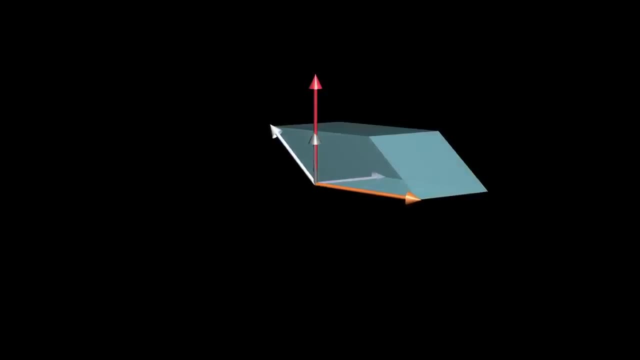 the dot product is negative will line up with the cases where the right hand rule for the orientation of x, y, z, v and w is negative. This means that we just found a vector that's perpendicular to the orientation of x- y. 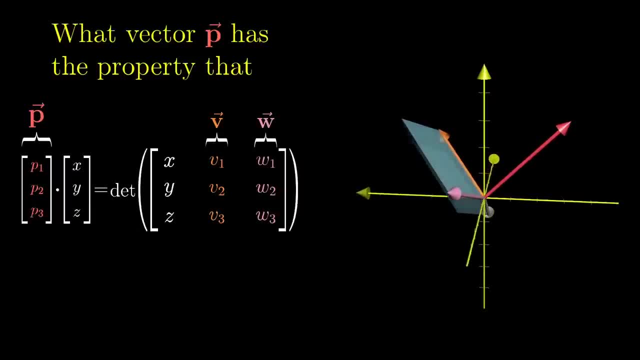 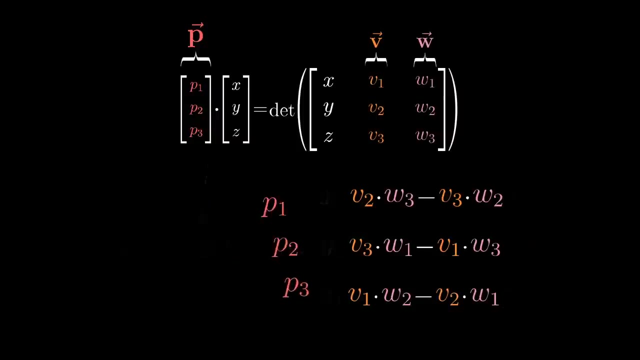 z, so that taking a dot product between p and some vector- x, y, z- is the same thing as computing that determinant of a 3x3 matrix whose columns are x, y, z, the coordinates of v and w. So the answer that we found earlier, computationally, using that special notational trick, must: 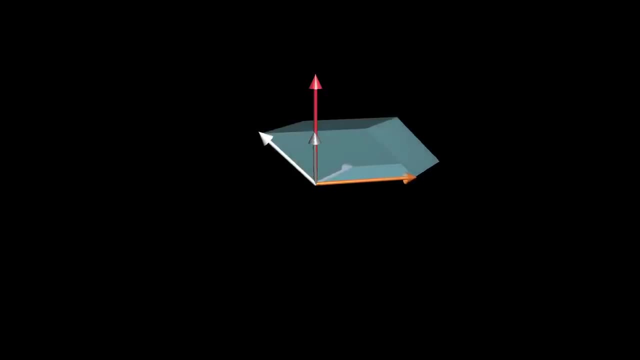 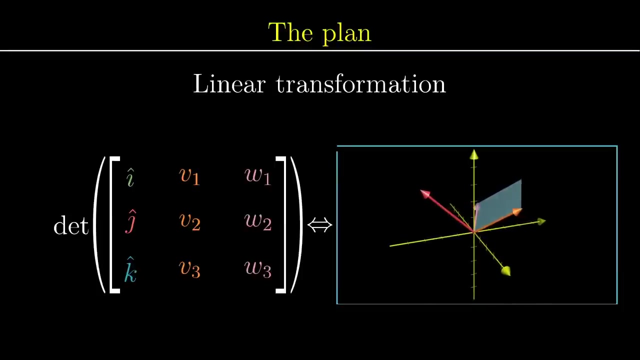 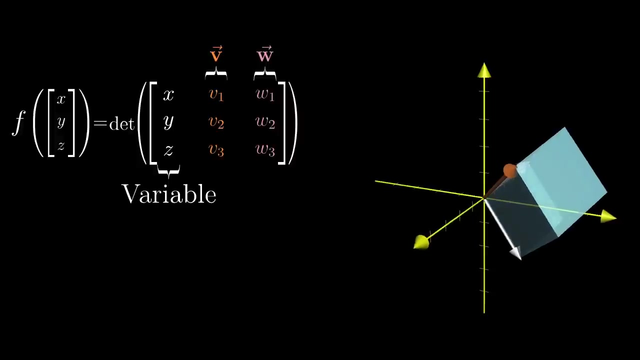 correspond geometrically to this vector. This is the fundamental reason why the computation and the geometric interpretation of the cross product are related. Just to sum up what happened here, I started by defining a linear transformation from 3D space to the number line, and it was defined in terms of the vectors v and w.